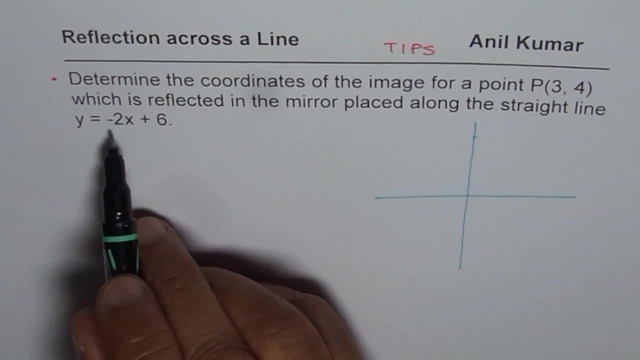 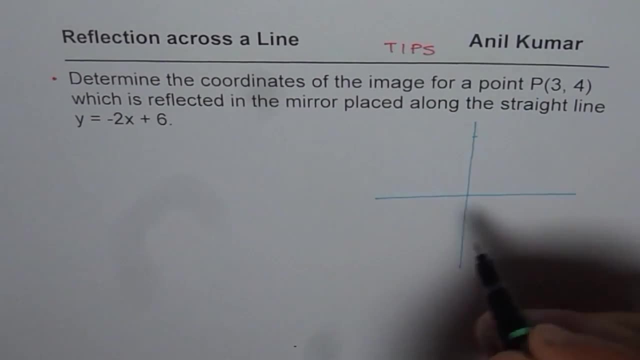 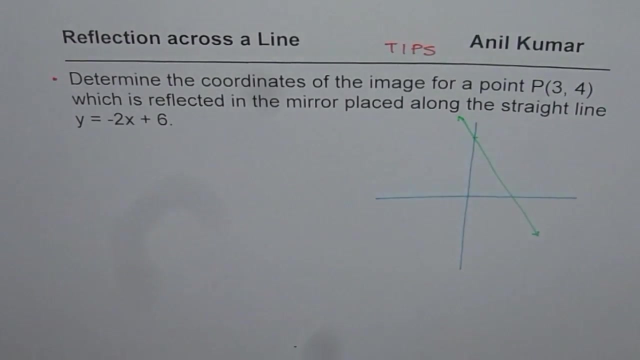 For us the y-intercept and slope is minus 2, so that means it is going downwards and this x-intercept will be at 3, right then, it gives you a slope of minus 2.. Let me first sketch a line here. So let this be the line which is with y-intercept of 6, and if this point is 3,, you know the slope is minus 2.. 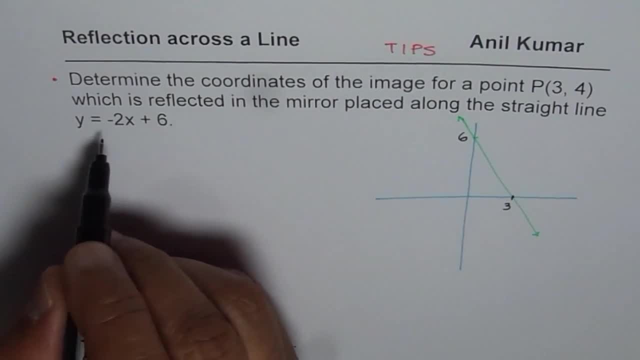 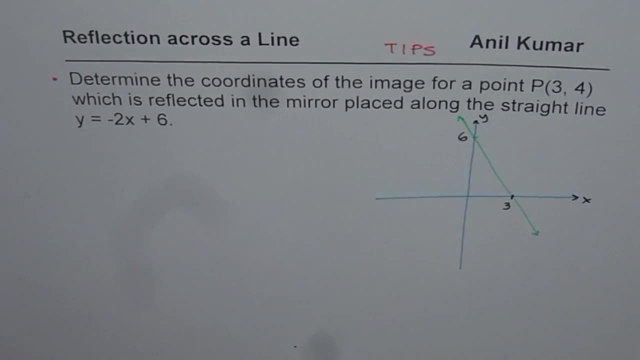 So that is the line for us. We will call this line as: y Equal to minus 2x Equals to. so let me say: this is y-axis, this is x-axis. Okay, Now we are given a point: 3, 4.. 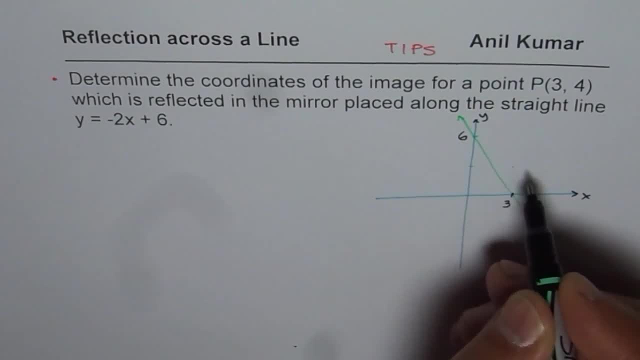 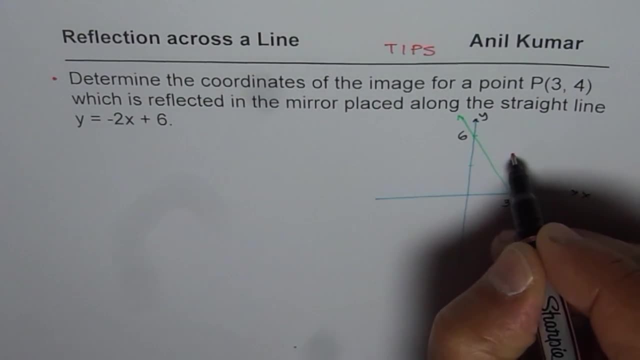 So approximately so. normally, as you find in my videos, we always use very approximate sketches which are good enough to give us just the right result. So we say 3, 4, is this point P right? so P is 3, 4 for us. 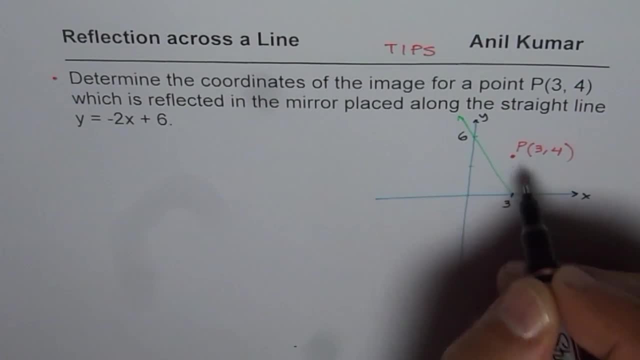 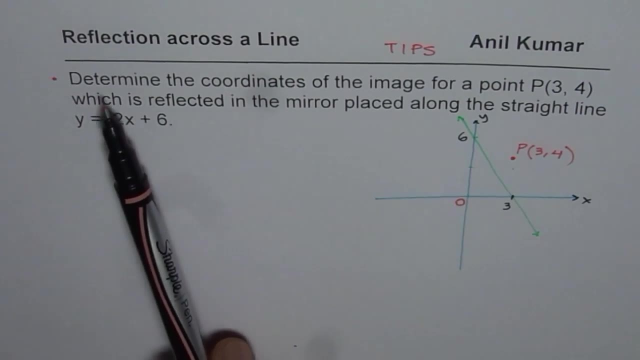 Right. so x value 3. Y value slightly more than half of this. Okay, so that is the origin for us. Now let us read the question once again. We need to determine the coordinates of the image for a point P, which is here, which is reflected in the mirror placed along the straight line. y equals to minus 2x plus 6.. 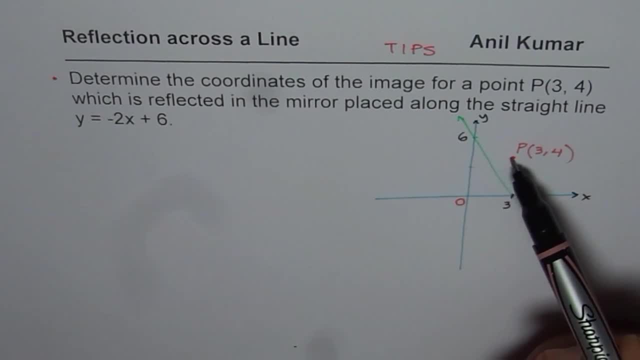 So this is the mirror for you. So it is reflected means it comes somewhere on this side. is that okay? So that is how the reflection is going to take place. So that is how the reflection is going to take place. So that is how the reflection is going to take place. 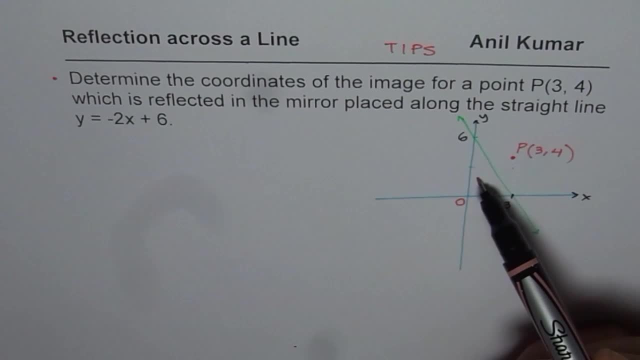 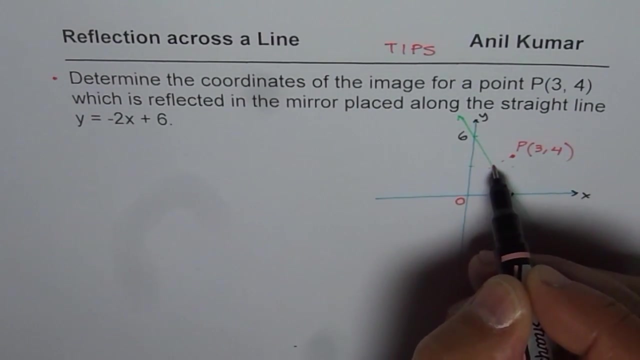 So we will find the image point coordinates. Now, how can you do that? Now, how can you do that? One thing which we all understand is that this mirror image is going to be at a distance which is same as in front of it, right? 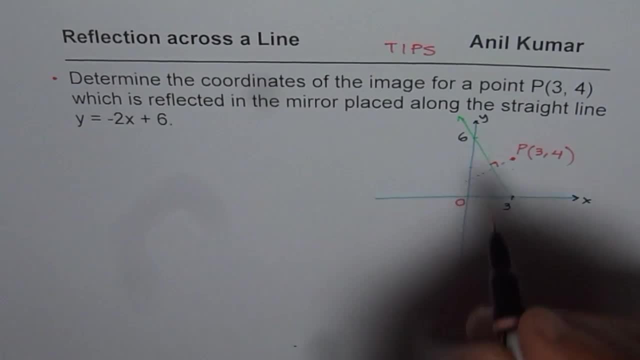 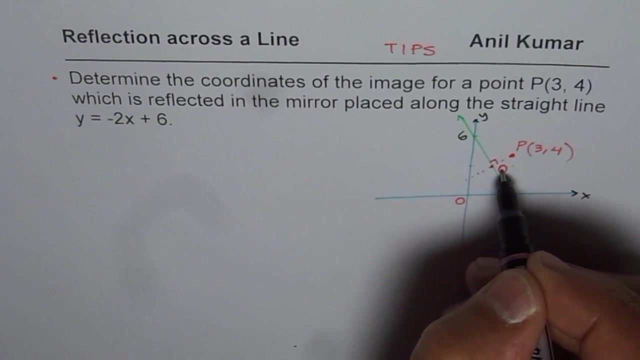 So that is the concept which we are going to utilize. So that is the concept which we are going to utilize. Let us say that, from P, we find a point on this line which is so that it makes a perpendicular to the line. So let me call this point as Q. 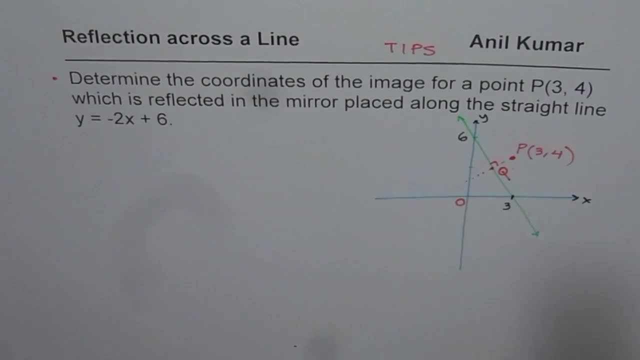 So we know PQ is perpendicular to the line. Let us say: line is L for us, So this is the line for us. Now we need to find this point Q on the line. Now we need to find this point Q on the line. 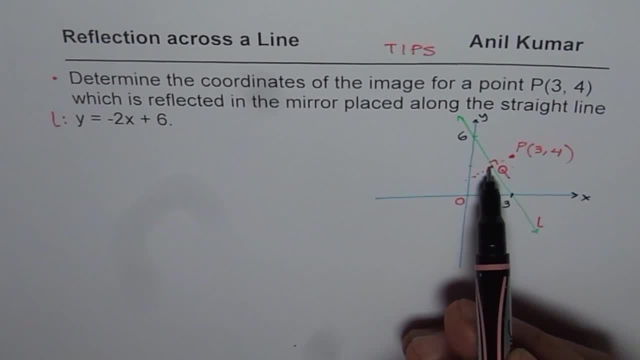 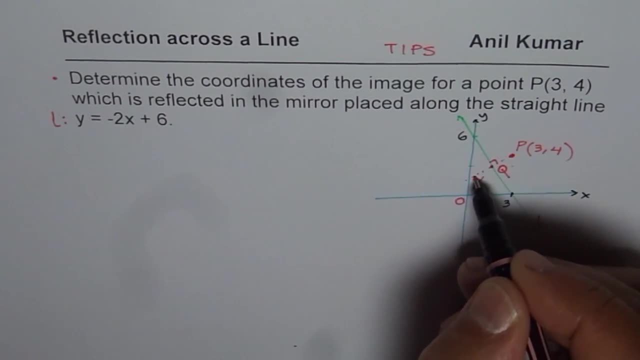 That will help us to get the image point which is as far behind Q as P is in front of it. You get an idea. So we are looking for a point, P dash this side And these two distances to be same. I hope you got the concept. 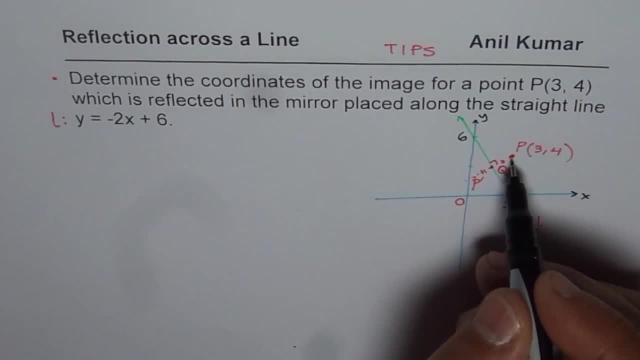 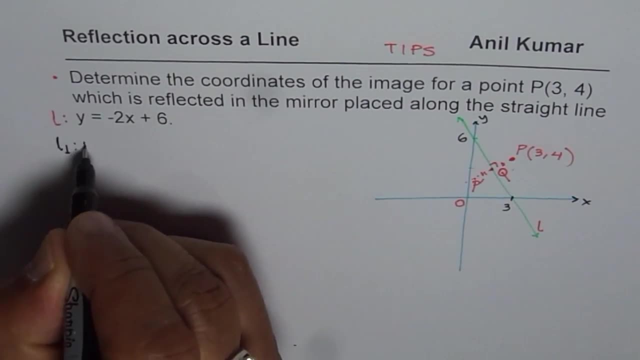 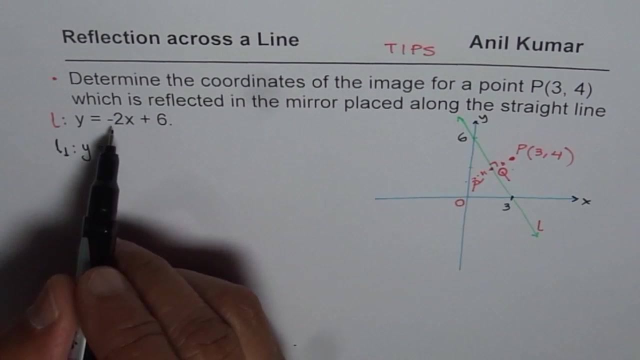 Correct Right. So what is the equation of the line which is perpendicular to the given line, L? So we say L which is perpendicular will be Y. equals to Slope should be negative reciprocal Right. So slope in our case will be, instead of minus 2, it is going to be half. 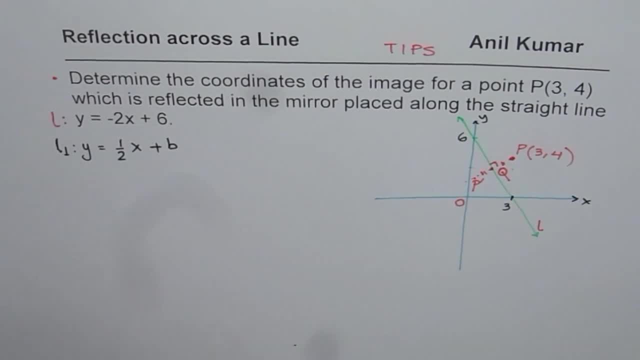 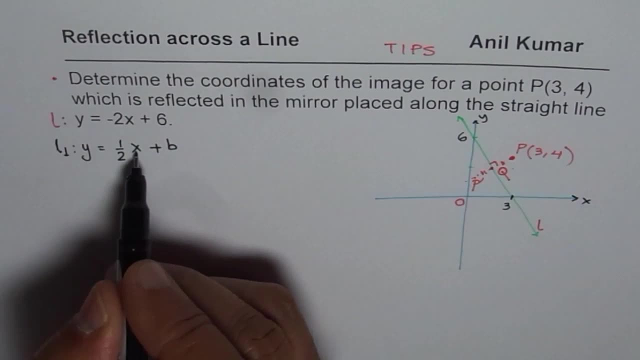 So it is half X And we do not know what B is. We will write B here. Now, since this line passes through the point, we will substitute 3 for X and 4 for Y. So 4 equals to half times 3 plus B. 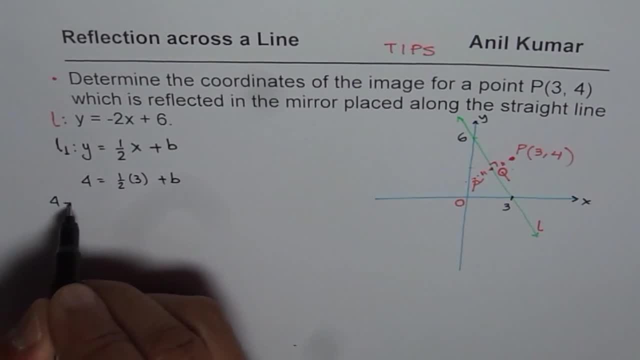 And from here we can find what B is. It is 4 minus 3 over 2.. And that is the value of B. So which is 8 minus? Let me write: 8 minus 3 over 2 is the value of B. 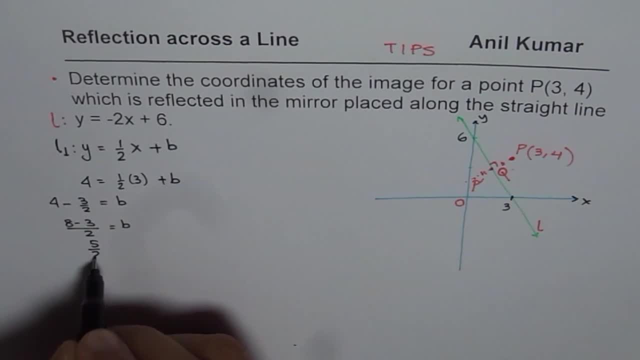 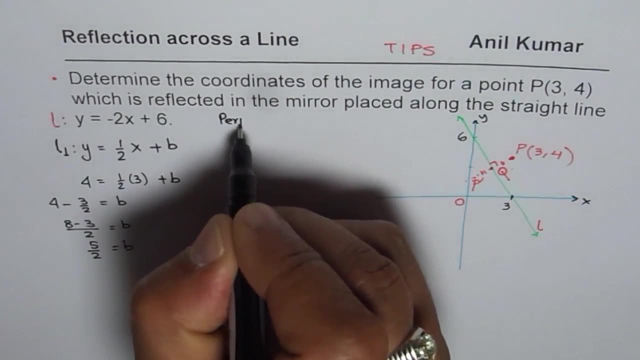 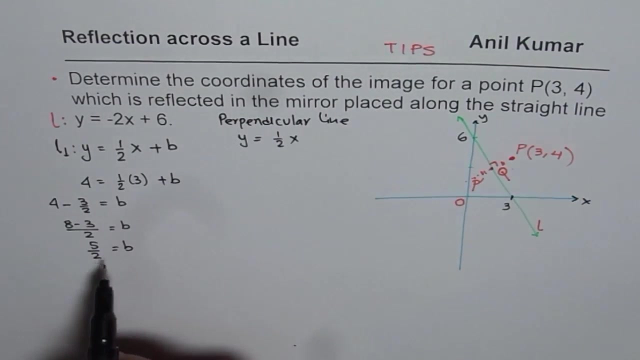 Right. Or we can say: B is equals to 5 over 2.. Right, So B is 5 over 2.. So that gives us the equation of a perpendicular line. So let me write down here now: Perpendicular line Will be: Y equals to 5, half of X and then Y values. 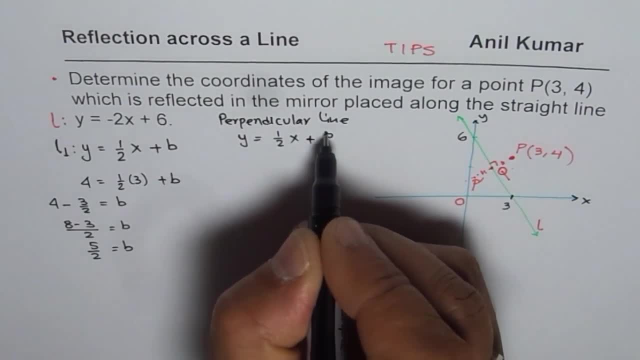 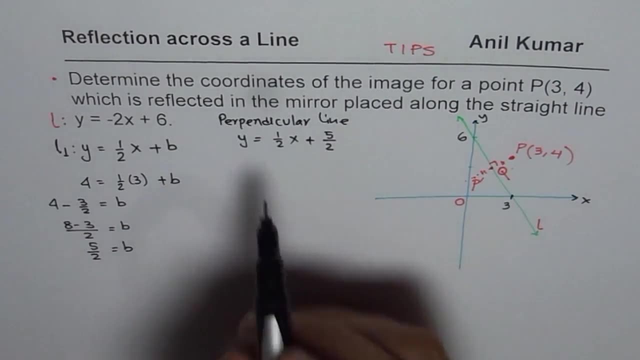 Y intercept is 5 over 2.. Or 2.5. Right, 5 over 2.. So that becomes the equation of the line. To write it in a simpler form, we can just multiply by 2 all these values. 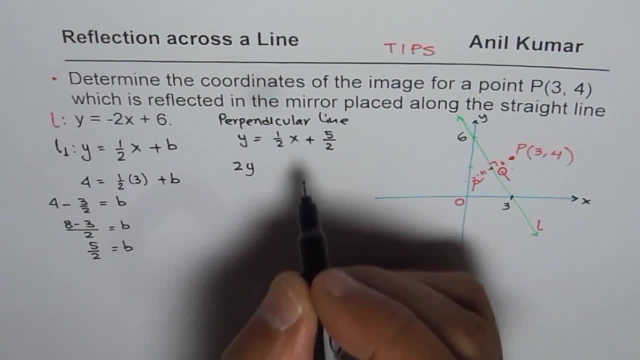 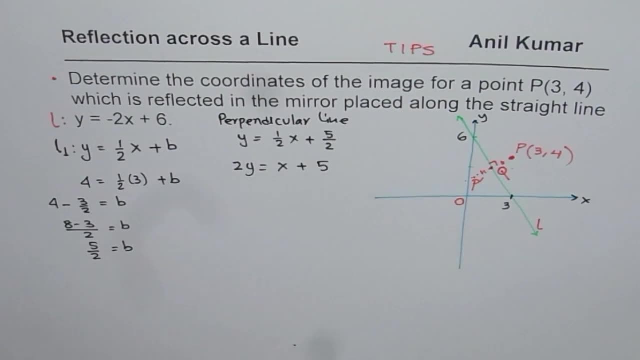 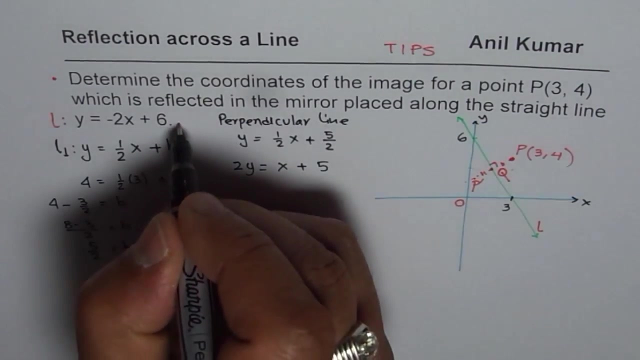 So we get 2Y, Or Okay, So 2Y equals to X plus 5.. So that becomes the equation of this particular line. Right Now we have two lines, So line 1 is Y equals to minus 2X plus 6.. 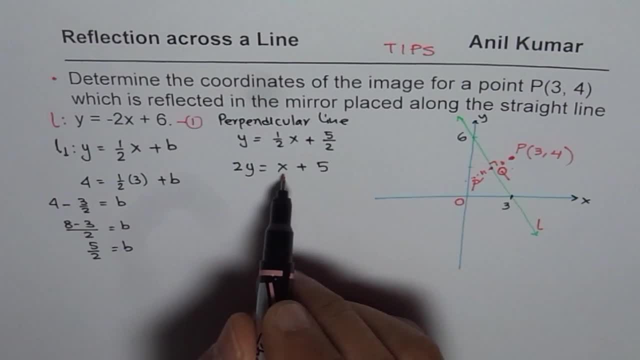 The line second one is 2Y equals to X plus 5.. So that is the second line. Now we need to find point of intersection, Which We could find using elimination or substitution. Let me write down what X is here, So we can say X is 2Y minus 5.. 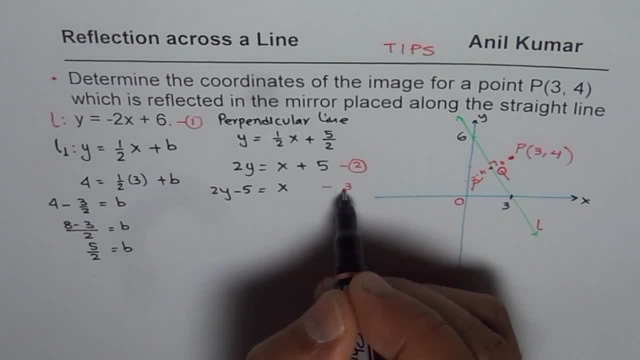 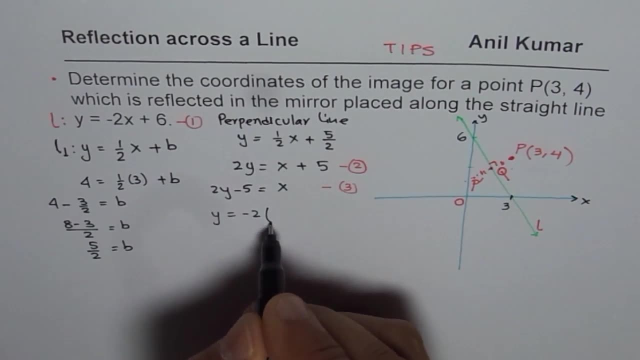 So we'll substitute this value of X in the given equation. So we say: Y equals to minus 2 times, So 2Y minus 5. That's the value of X Plus 6. Right, So that gives us minus 4Y. 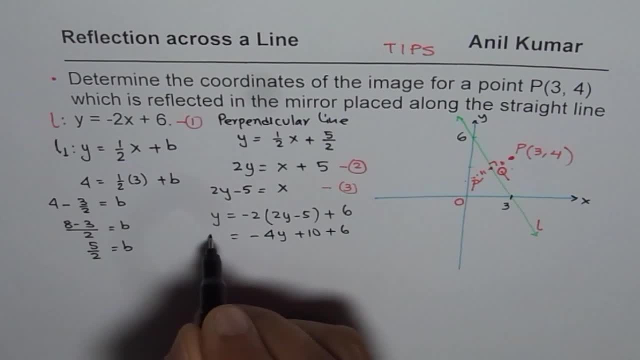 Plus 10.. Plus 6. Equals to Y. Bringing it to the left side gives us 5Y equals to 16. Or Y equals to 16 over 5.. So we get the Y value as 16 over 5.. 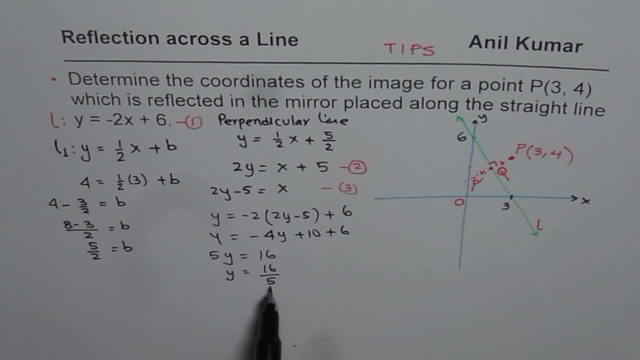 Once we know the Y value, we can find the value of X Right. So what is X equals to? X is equals to 2Y minus 5.. So 2 times 16 over 5 minus 5.. That is what we have. 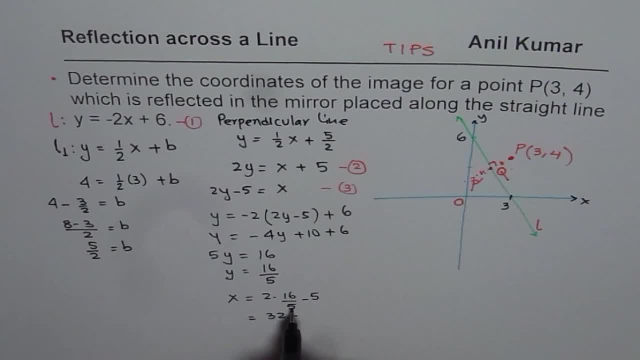 So that is 32 minus 5 times 5 is 25 divided by 5. Or that is 7 over 5.. So we get these coordinates for Q. So let me write down the coordinates for Q now. So the coordinates for Q are: 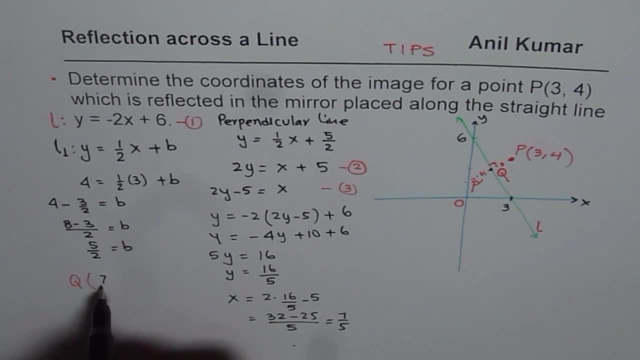 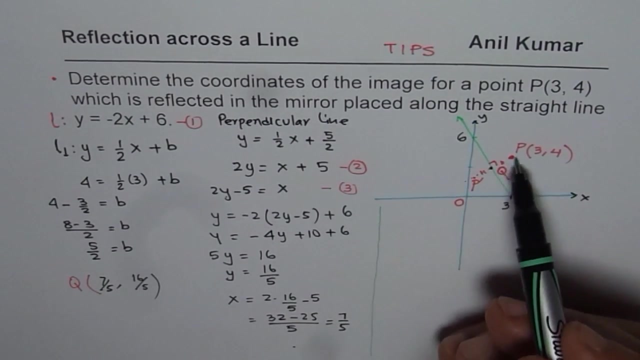 X value is 7 over 5.. And the Y value is 16 over 5.. So that is the coordinate of Q. Now the difficult part of the question is to find the coordinates of P', which is on the other side of Q. 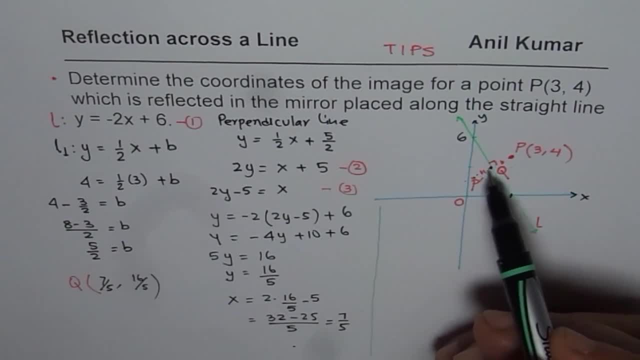 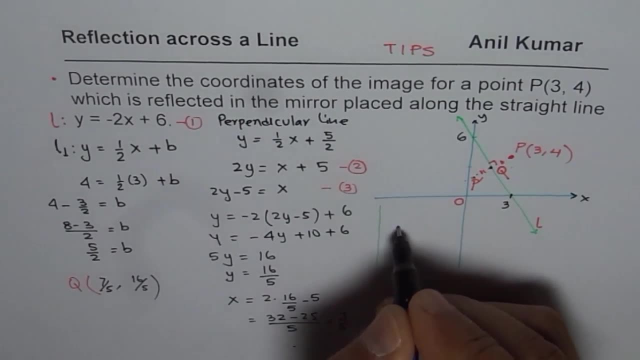 How do you find that Now we know Q is the midpoint. Since Q is the midpoint and we don't know what coordinates of P are, let us assume that the coordinates of P' are X and Y, Since Q is the midpoint. in that case, 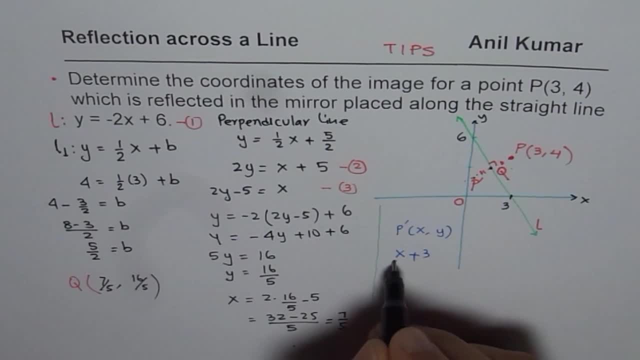 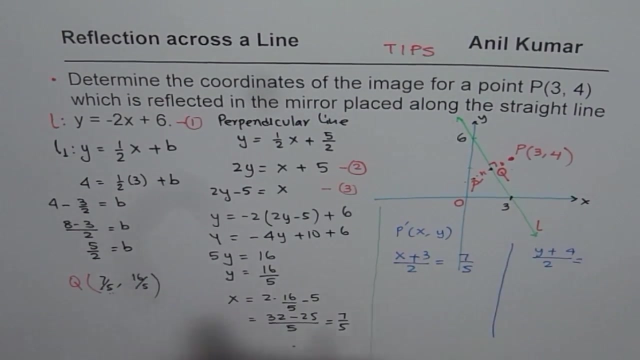 X plus 3, divided by 2, should be equals to the coordinates X value of Q, which is 7 over 5.. And the Y value should be: Y plus 4 divided by 2 should be equals to the Y value, which is 16 over 5.. 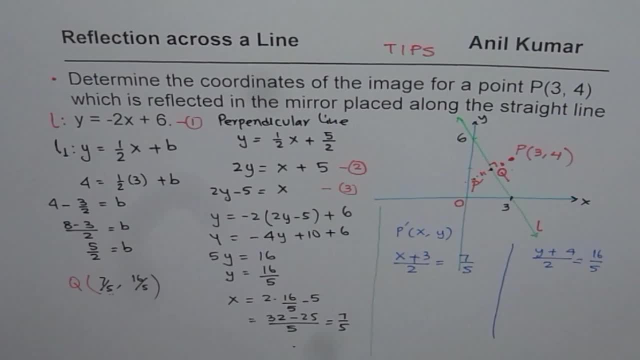 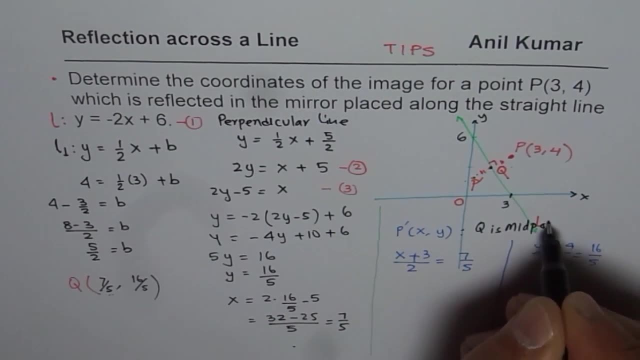 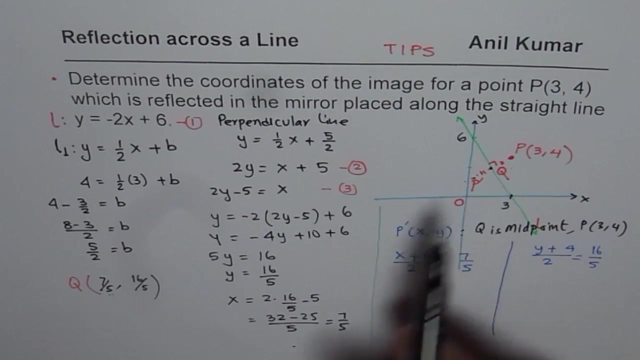 Do you get an idea Right? So what we have done here is we know Q is the midpoint, So Q is midpoint, Since Q is midpoint X, midpoint of P' and P, which is 3 comma 4, so X plus 3 divided by 2 should be equals to the Q value. 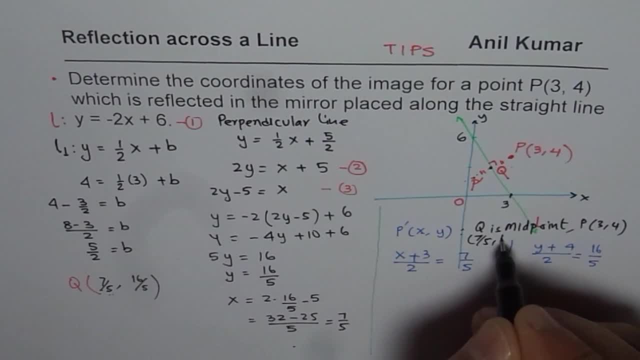 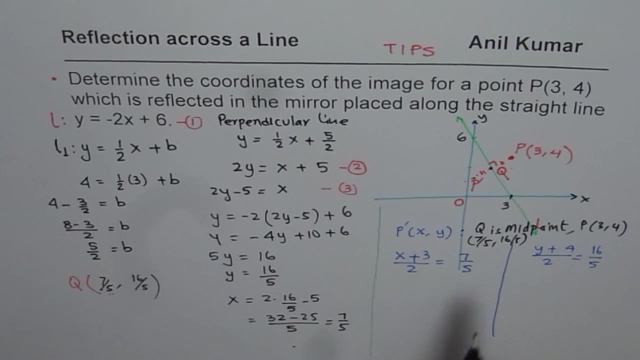 which is 7 over 5.. Let me write here: 7 over 5 and 16 over 5.. Correct, So we get two different equations, and these equations will give us the value of X and Y. So let's cross, multiply and then find. 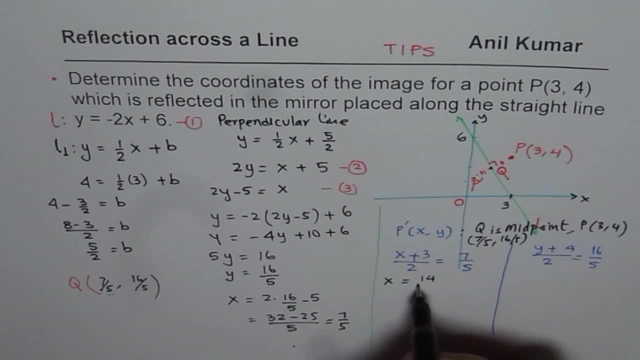 So we have X equals to: when you cross multiply, you get 14 over 5, and then we take away 3, minus 3.. So we have 14 minus 15 over 5,, which is minus 1 over 5.. 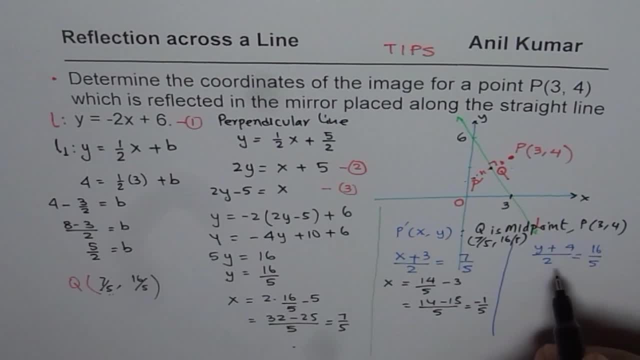 That is the X value, And as far as the Y value is concerned, we'll have: Y plus 4 equals to cross multiply 32 over 5, or Y is equals to 32 over 5 minus 4, which is 20, right. 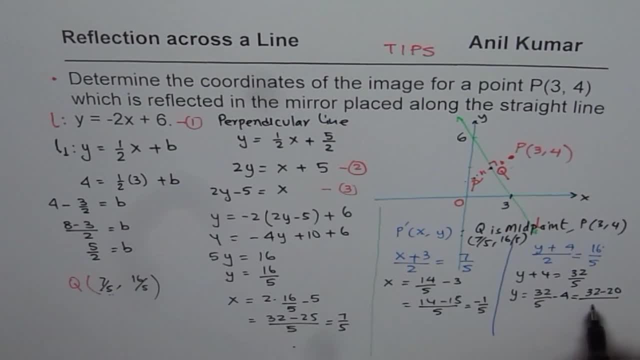 32 minus 20 over 5,, that is equals to 12 over 5.. So 12 over 5 is the Y value, right? So approximately that is. I mean I'm not writing approximate, We are writing in fractions itself. 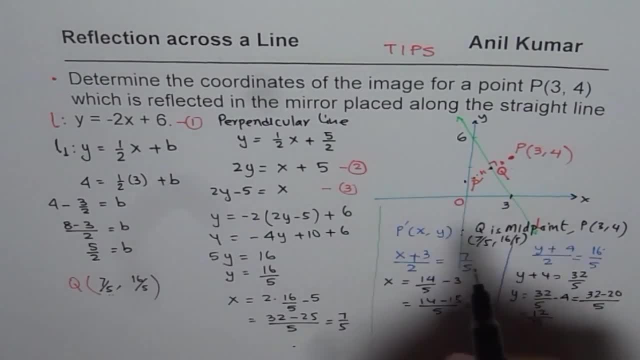 So what we get here is, the point is slightly on the left side of the Y axis. So we say: image is P, dash, which is X value is minus 1 over 5, and Y is 12 over 5.. So that becomes our answer. 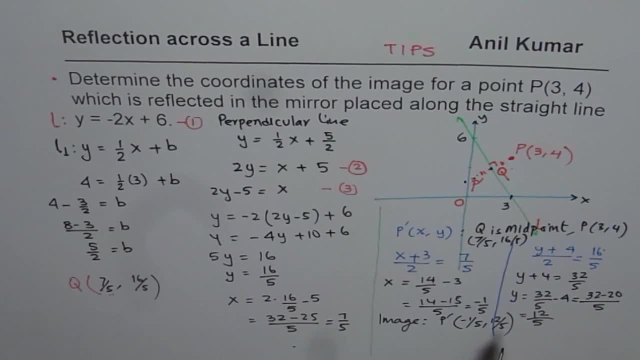 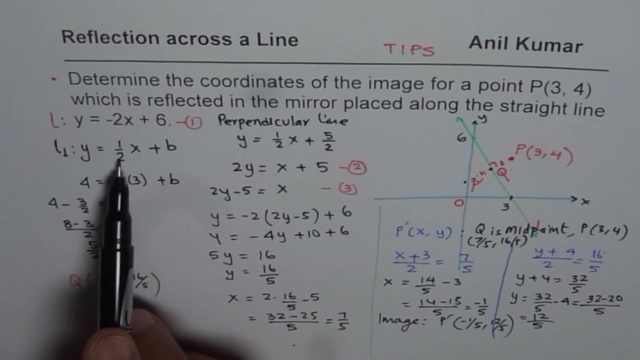 You get an idea. So the steps involved are: first: 0.34 will lie on a line which is perpendicular to given line, right, So this line is perpendicular. Slope of perpendicular line is negative, reciprocal. So we got the slope as half. 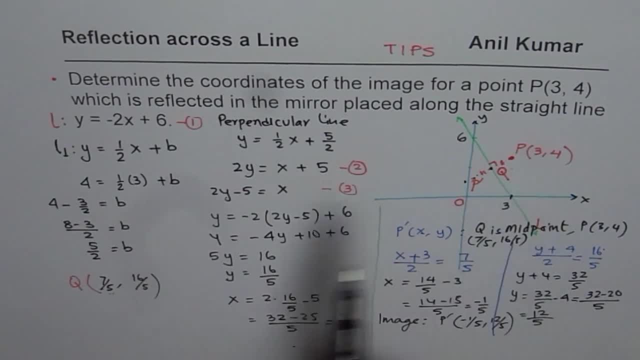 Now find B using the given 0.3 and 4.. Once you get the equation of the perpendicular line, now we need to find intersection of these two points right. So we found, at this stage we are trying to find intersection, right. 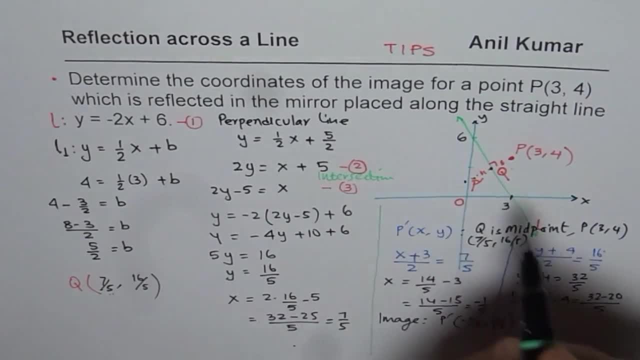 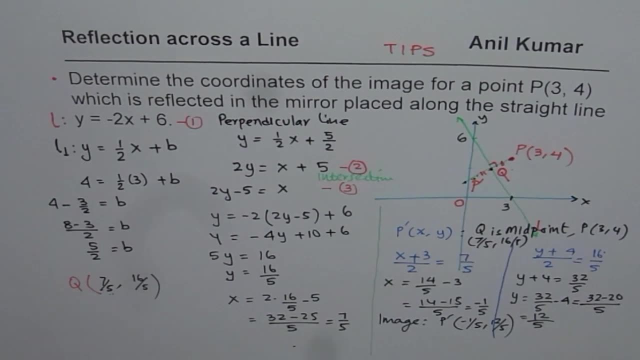 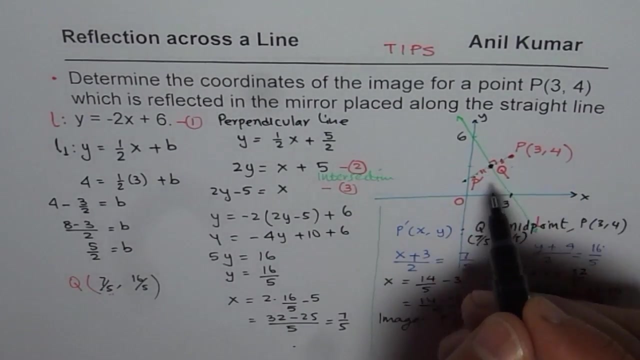 So intersection of the two given lines, these two lines, correct, That point of intersection is actually the midpoint between the point P and its image Right Now. so once you find the center point Q then, which we found as 7 over 5,. 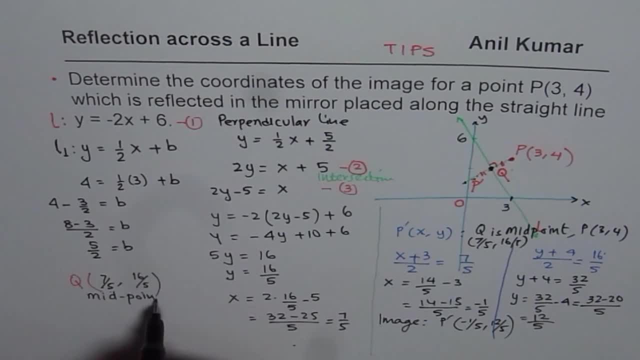 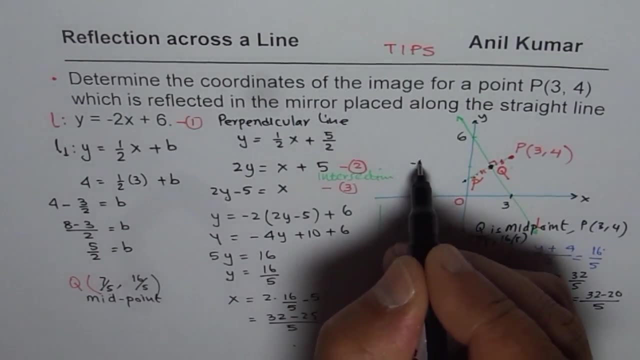 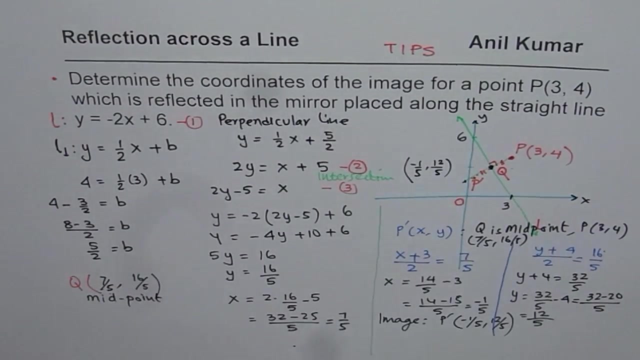 that is the midpoint right. Then use the midpoint formula to find the image point. So we found the image point as minus 1 over 5 is the X value and 12 over 5 is the Y value, right? So that is how you do it. 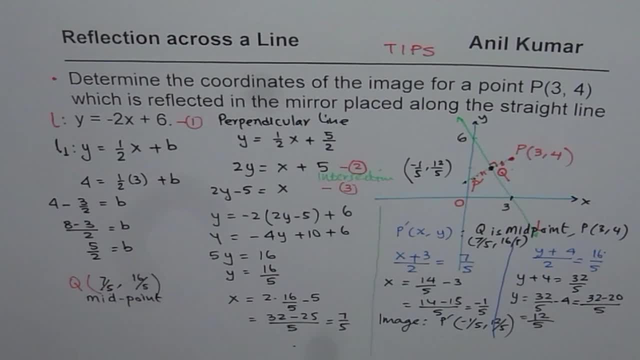 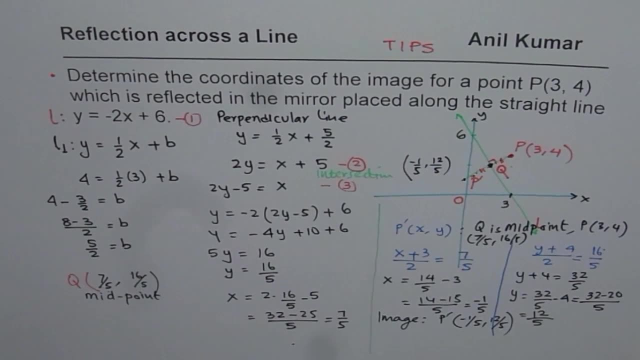 I hope you understand and appreciate the steps. We'll take few more examples to help you develop this concept. Thank you and all the best.